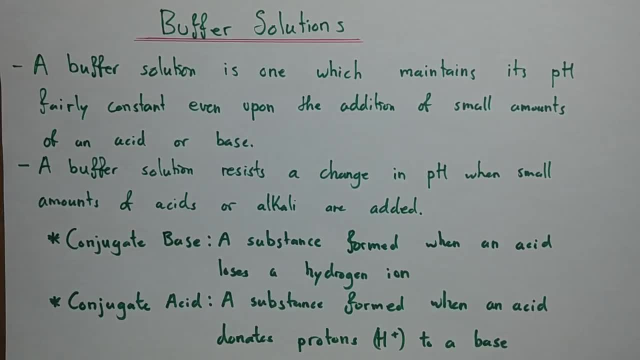 conjugate acid. So we see how those two are used. Conjugate base is simply a substance formed when an acid loses a hydrogen ion, while the other is a substance formed when an acid donates protons to a base. Okay, so from there let's see what happens. 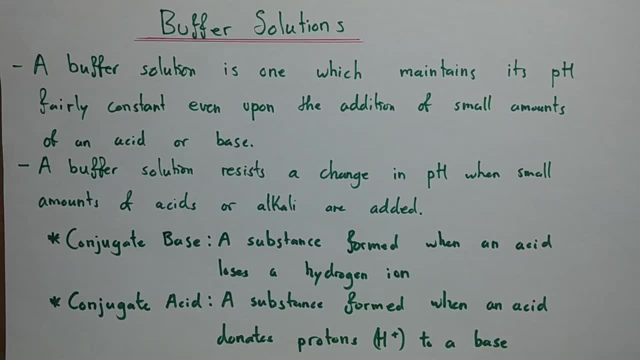 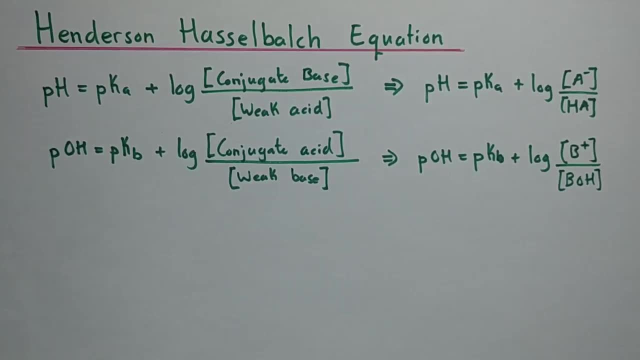 Let's see how we can break down this concept of buffer solutions. Okay, so there are some equations we're going to be looking at. These equations are known as the Henderson-Hazelbach equations. So the main equation or equations for this scientist is the one which you get: the pH. The pH is given by the pKa plus the log of the conjugate. 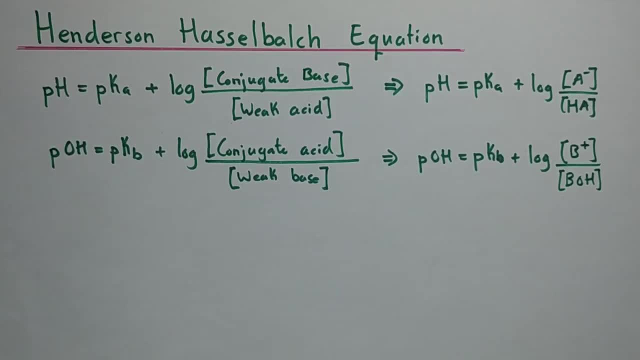 base of a weak acid. So a conjugate base is usually given the symbol A minus and the weak acid is given the symbol HA, while the potential of the hydroxyl gives you the potential of the base association constant plus the log of conjugate acid divided by conjugate base. Okay, so there. 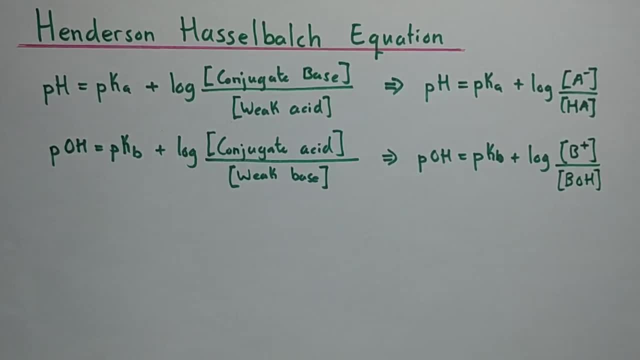 are some other useful formulas that we can use in the process of calculating what we're going to be finding. Okay, so, to start with, how do we find the acid association constant? So one thing you should know about the acid association constant is that it is given by 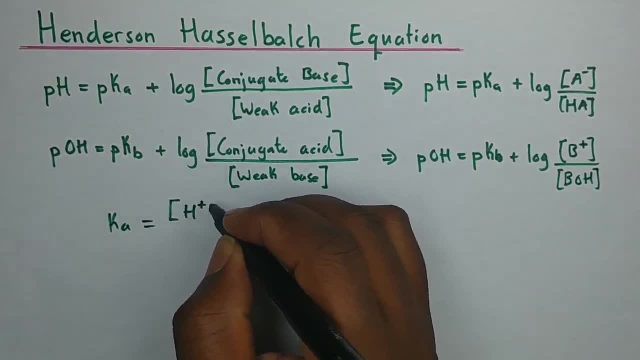 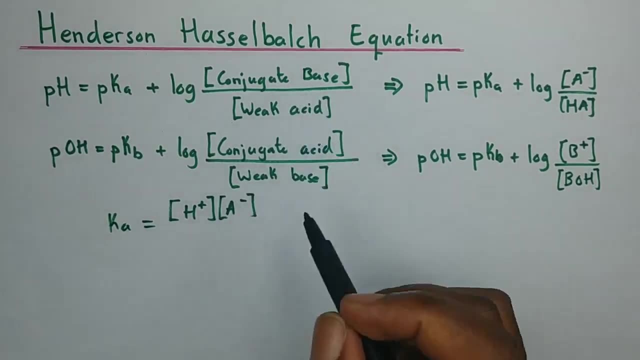 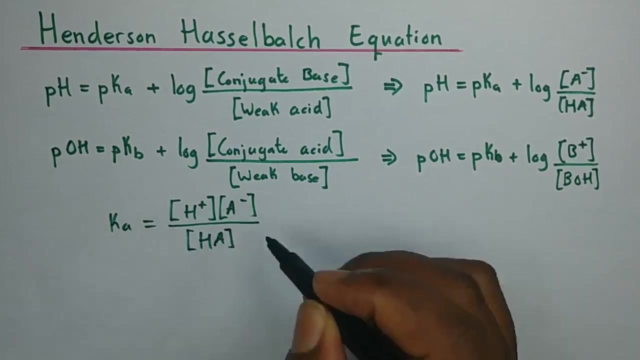 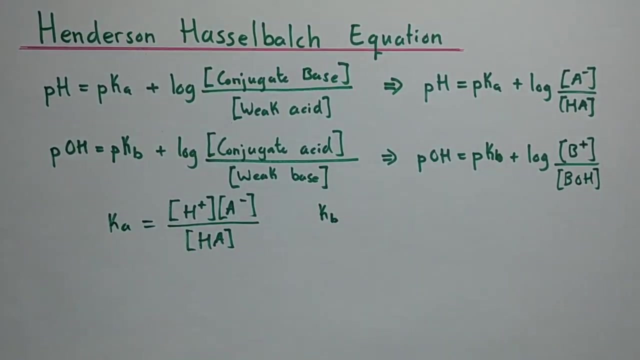 the concentration of H, which is the hydrogen plus A minus, which is the concentration of the conjugate base divided by the pKa. Okay, Then we also have the constant association of the base, Similar to this one. it is given: 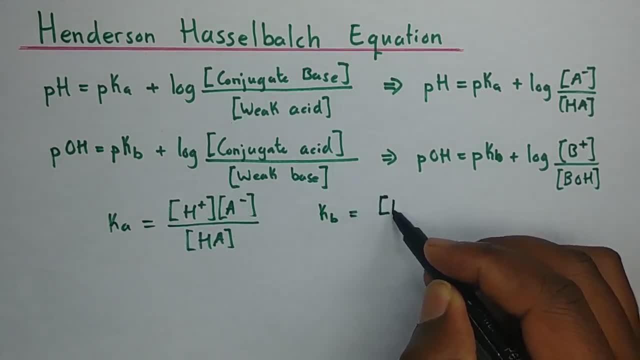 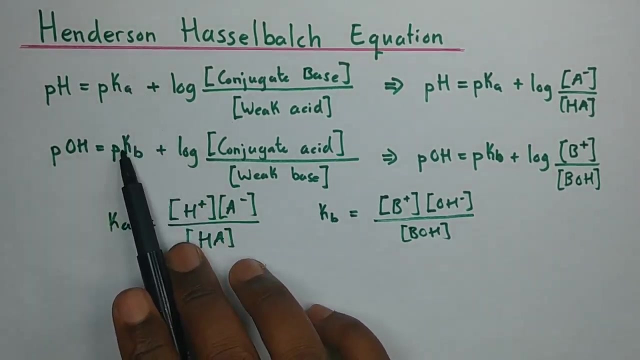 by B plus. B plus is simply the conjugate acid multiplied by the hydroxyl, and everything is divided by the B or H, Okay, which is the weak base. okay, so now, from these, they can be used to find the PKA and the PKB. remember, we found PKA, we found PKB. we can use these to find. 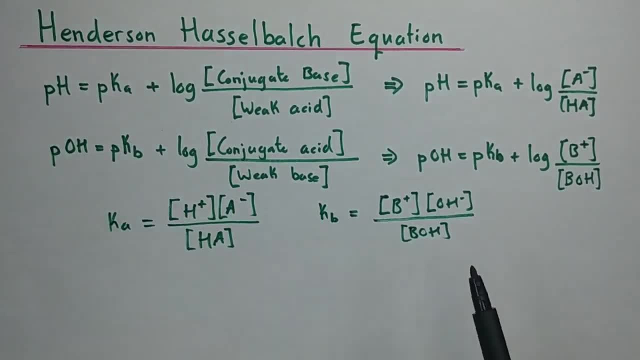 the PKA. right here, we just have the KA and the KB. rather so to find the PKA, the PKA, or let's start with the pH, first of all, one thing you should know about the pH is that the pH can also be found by equating this to a negative log of the. 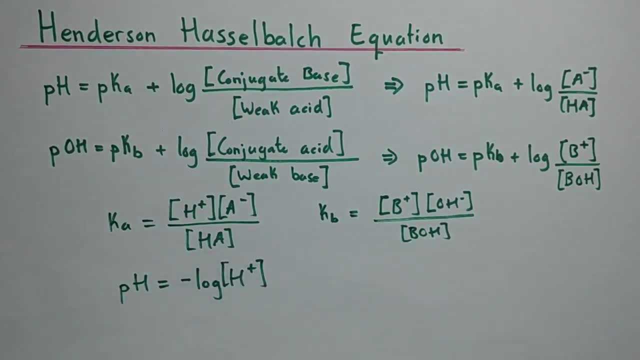 hydroxyl. not the hydroxyl, rather the hydronium, because we are looking at hydrogen. then for the pOH: pOH is found by a negative log of the hydroxyl. now. okay, so this is a negative log of the hydroxyl now. so this is a negative log of the hydroxyl now. 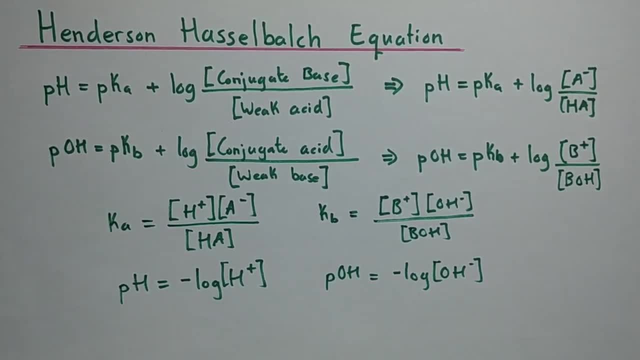 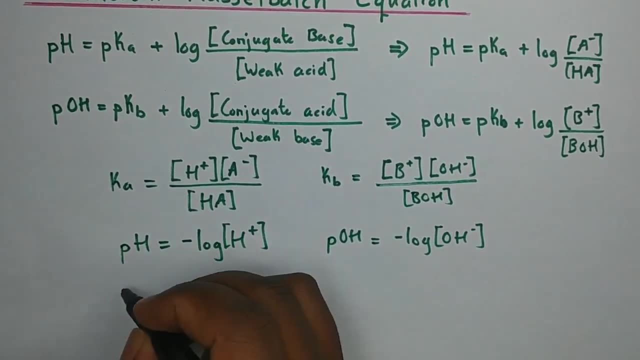 so we have the hydrogen and the hydroxyl, but in this case we're looking for the PKA and the PKB. so we'll see that the PKA- PKA- is given by the negative log. same thing. negative log, then the concentration of the acid association. 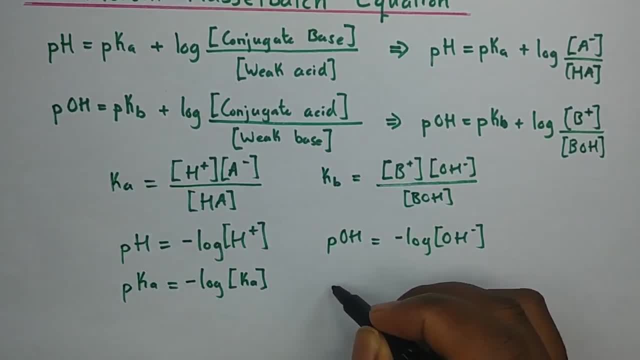 constant. same thing applies. the PKB is found by the negative log of the concentration of the P, or rather the KB, which is the constant of the base. so these are just some useful formulas that you need to know as we look into this topic. so let's go ahead and look at an 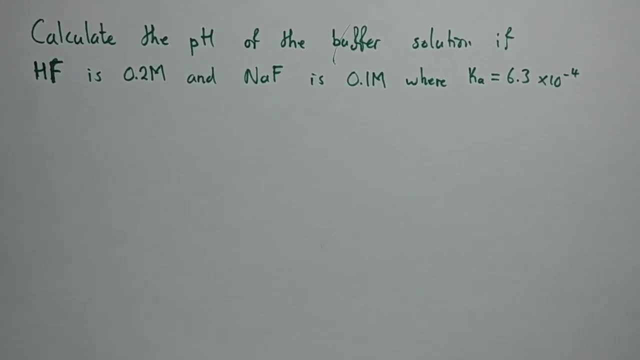 example. okay, so in our first example we're going to have to calculate the pH of a buffer solution. if HF is equals to 0.2 molar of NaF, which should be sodium fluoride is 0.2, where the acid associated constant is 6.3 times 10 to the power negative 4.. Okay, so let's see. 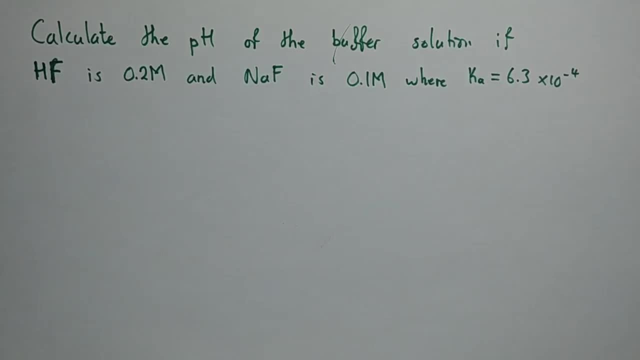 what we have. let's analyze the question. first of all, We need to know which one is our base, which one is our acid, which one is our conjugate, and everything, so that we see how we can use that to find the pH, The formula we're going to use to find the 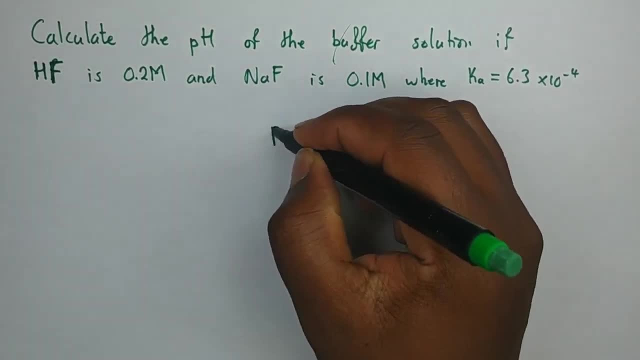 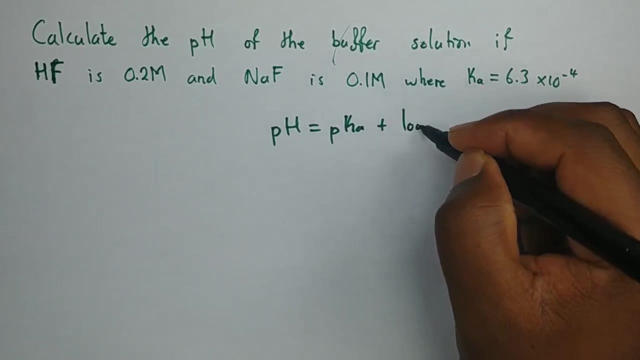 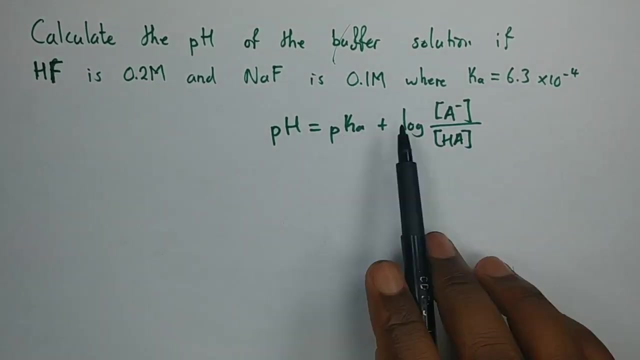 pH is. the pH is equal to the pKa plus the log of the conjugate base. it's a concentration divided by the concentration of the weak acid, like that. So now all we need to know is we need to find our pKa, we need to know our base. we also need to know our acid. 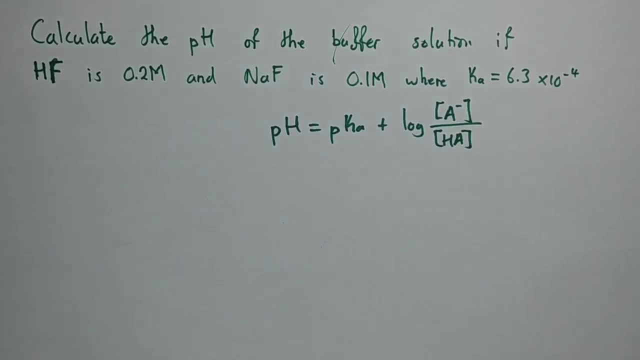 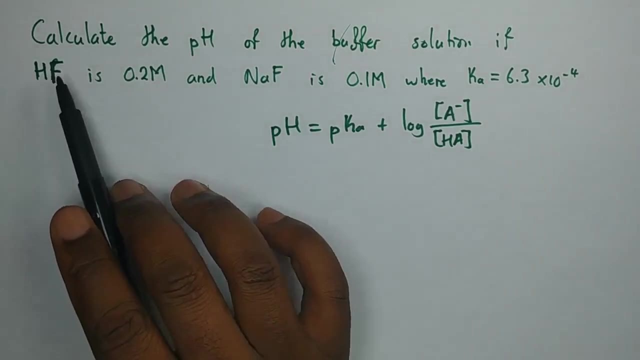 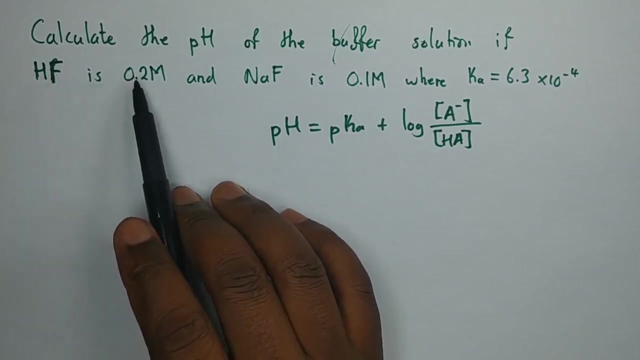 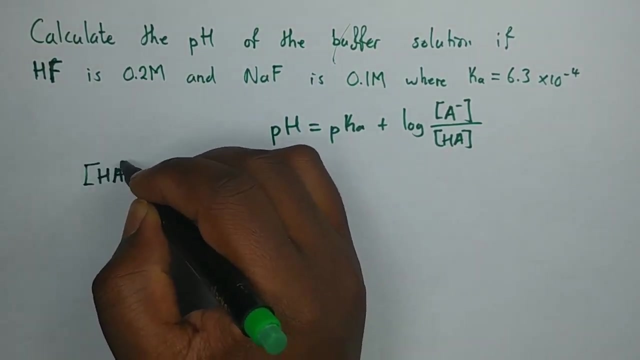 So, from the question we need to analyze which one is our base, This that we have here- hydrogen fluoride, you can call it, is our acid and it is given a concentration of 0.2.. So, since an acid, or a weak acid rather, is given the symbol HA and you can say: 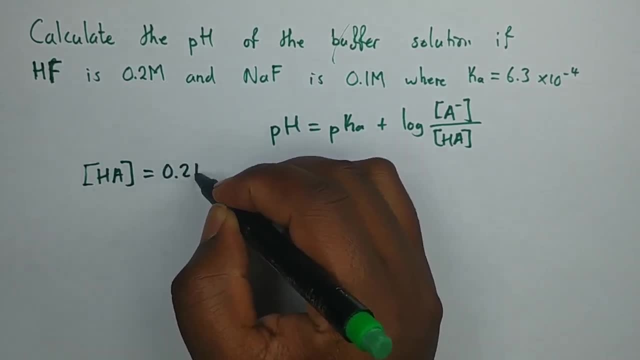 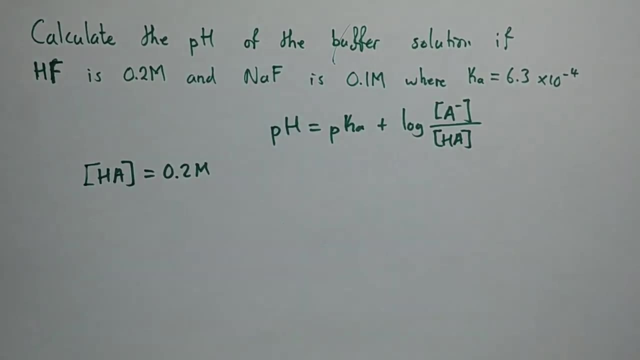 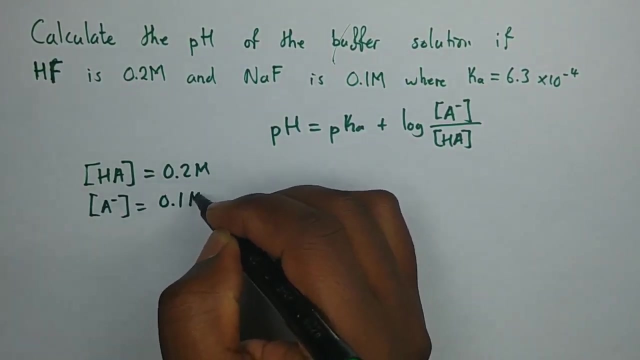 the concentration of HA is simply equal to 0.2 molar. Then the concentration of the base, the conjugate base in this case. so concentration of the base is given by 0.1 molar, like that. Then now we just need to find the pKa. We do not have the. 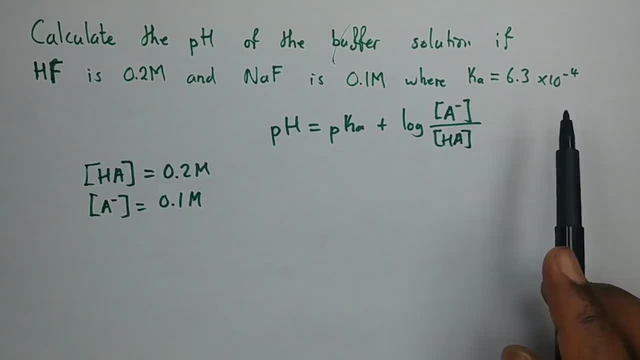 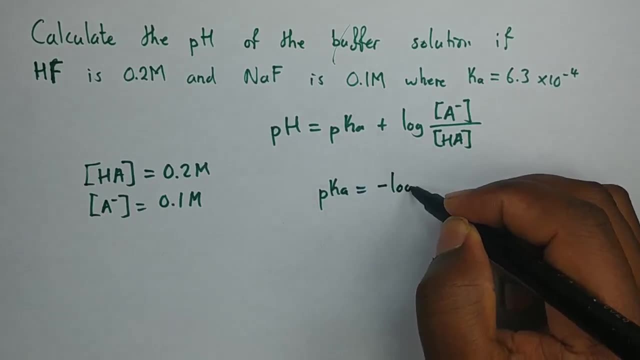 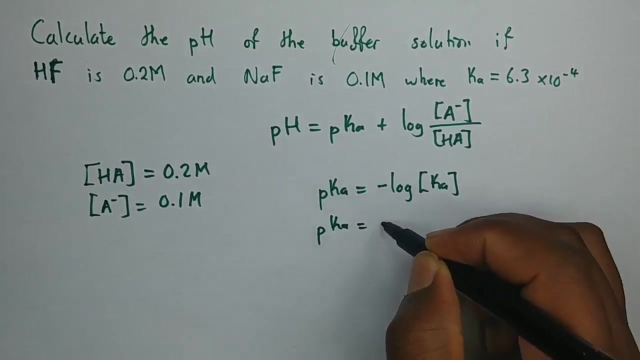 pKa, but rather what we have is the association constant. So from this we know that the pKa can be found by negative log of the Ka. So to find the pKa, I'm going to say negative log- the Ka is this value, that 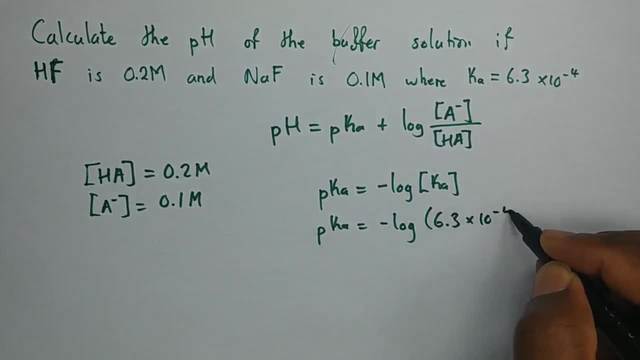 we have here, which is 6.3 times 10 to the power, negative 4.. So the pKa is usually, or rather the Ka is usually, given in the equation. So if we compute for the pKa, the negative log of this whole value that we have here, we're going to find that our 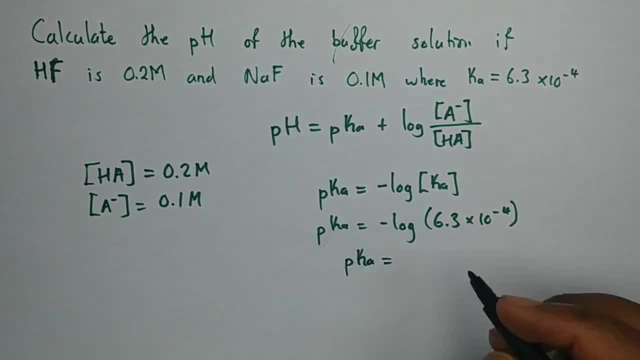 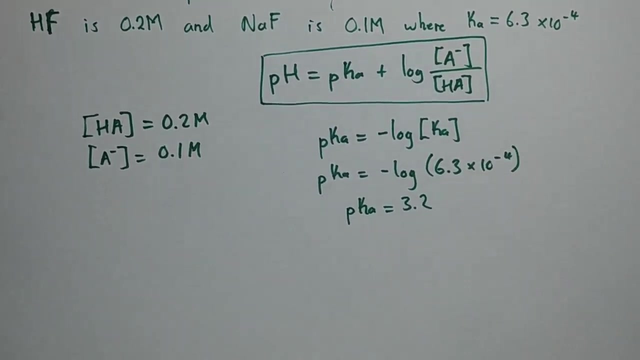 pKa is equal to 3.2 molar. okay, so what we've found is just the pKa. so now we're going to get everything that we have to replace in this formula because, remember, we're looking for the pH, so the pH is equals to the. 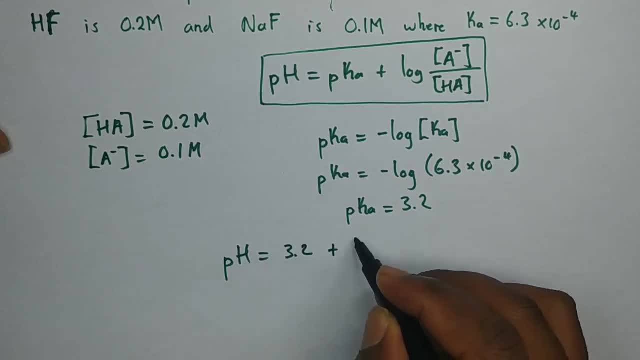 pKa we've found 3.2 plus log of A minus is 0.1. so that's 0.1 divided by HA. the weak acid is simply 0.2. okay, so the pH. let's see what this gives us. so the pH is given by 3.2, the whole thing here. 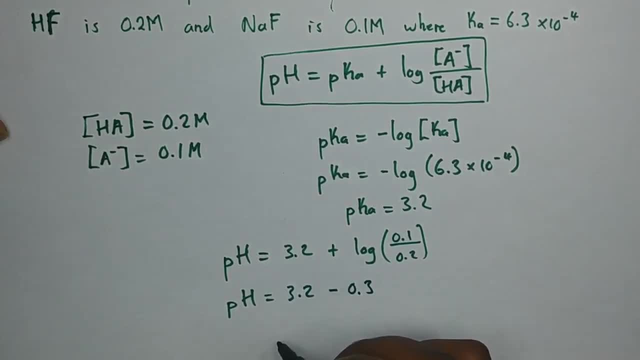 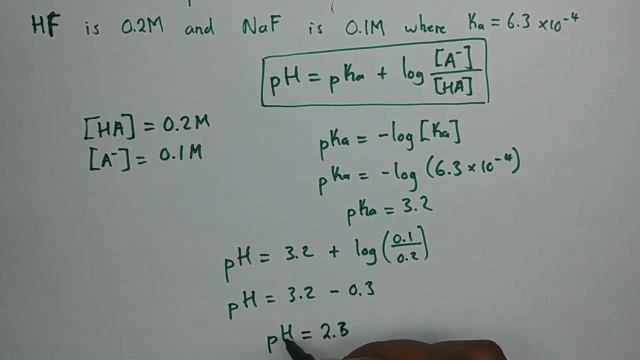 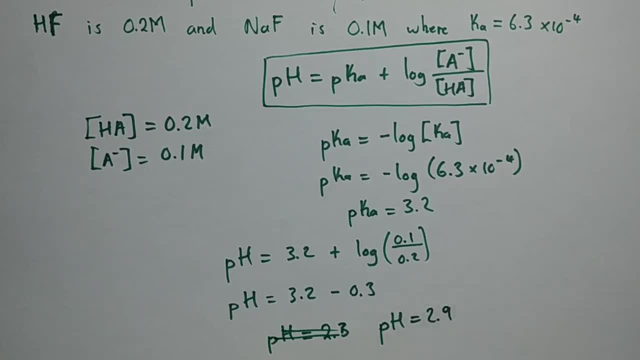 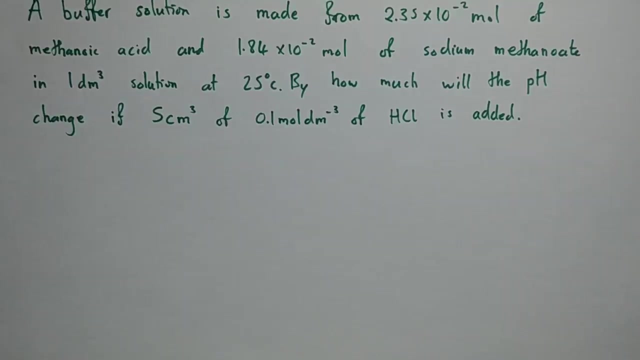 is equals to 2.9. okay, so that's how we find the pH for such equation. let's look at another example so that you can see how it actually works out. okay, in this example, well, we have a buffer solution that is made from those number. 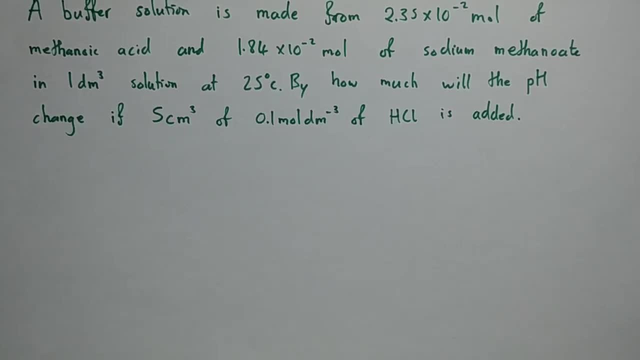 of moles of methanoic acid and those number of moles of sodium methanoate in one cubic decimeter solution at a temperature of 25 degrees Celsius. by how much will the pH change if five cubic centimeters of 0.1 more per decimeter? 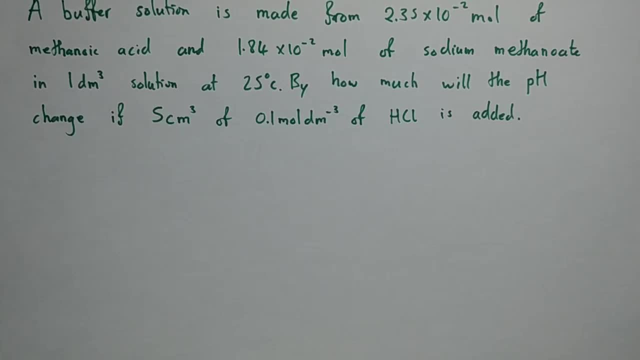 or per cubic decimeter of hydrochloric acid is added. so we have a scenario where you have this solution, then you add an acid- a strong acid for that matter- which is hydrochloric acid. then the acid for how much will it change? meaning that we need to calculate for two pH, one pH. 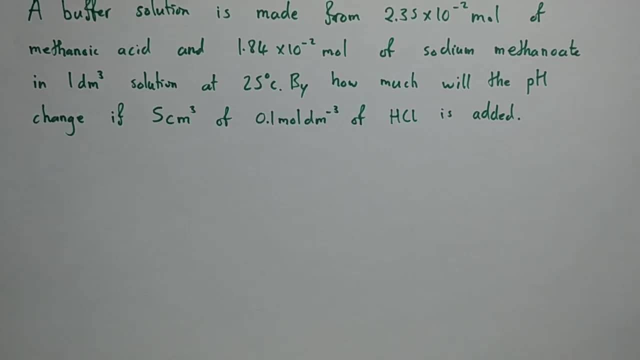 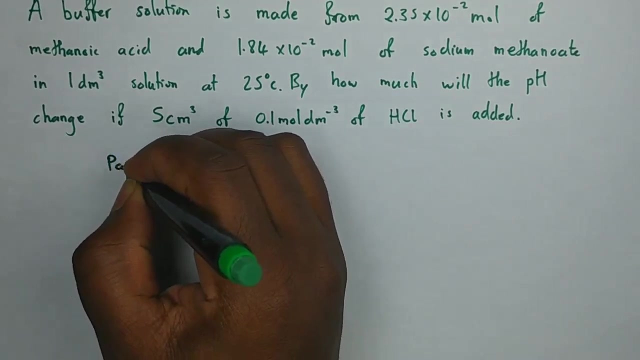 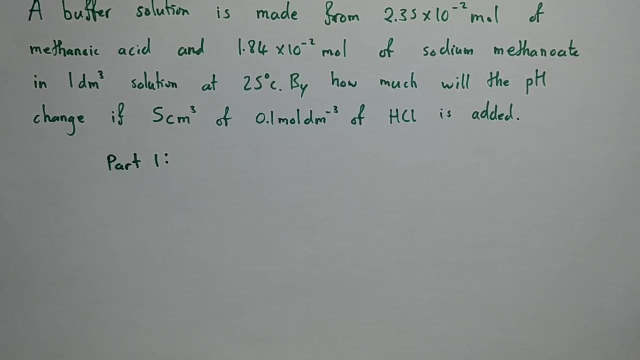 without the acid, or rather without the strong acid and the other pH when added, when the acid is being added. so I want to do it in two parts. so this is what we have, part one. so in part one. one thing you need to know about what we have here is that we do not have, or have not been given, any constant. so 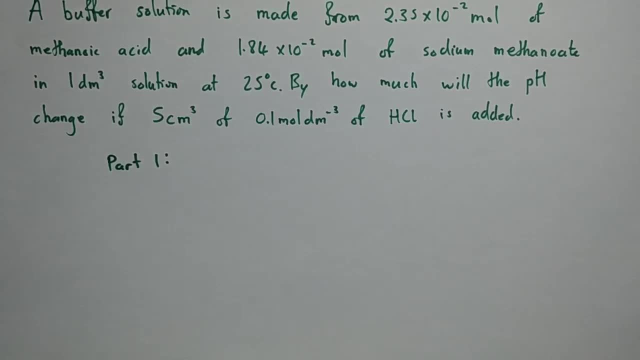 far as we can see in the equation, a constant has not been given to us, but one thing you should know about the solution that we have in this case is that it has a constant of 3.75 as the pKa. so that is for the acid, the. 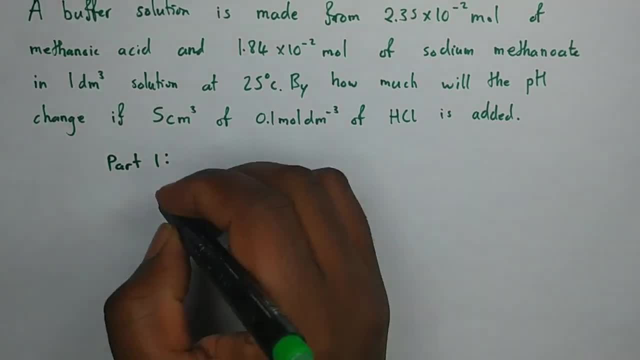 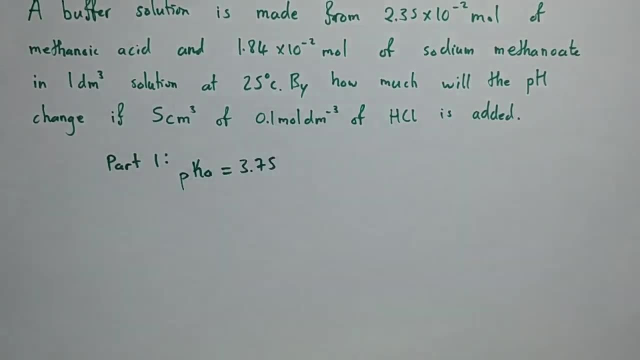 potential of the acid dissociation constant. so the pKa is given as a standard value to be 3.75. so that is just something that you have to know. so from this value we can actually calculate for the Ka. so with a Ka, once we've prepared for the Ka, then we can see how we can find the pH. but the Ka in. 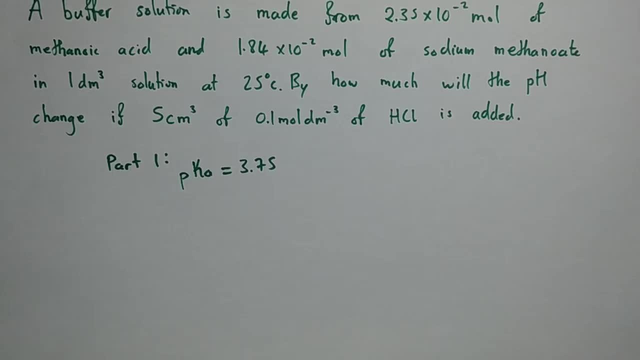 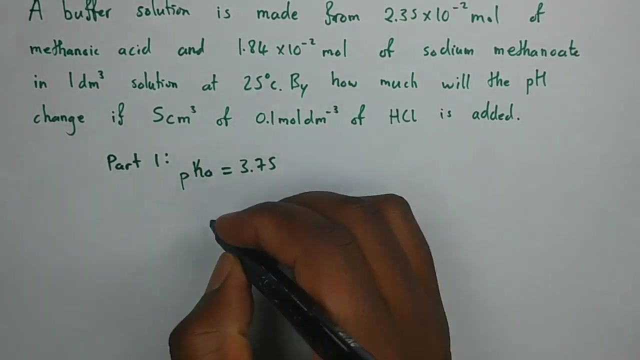 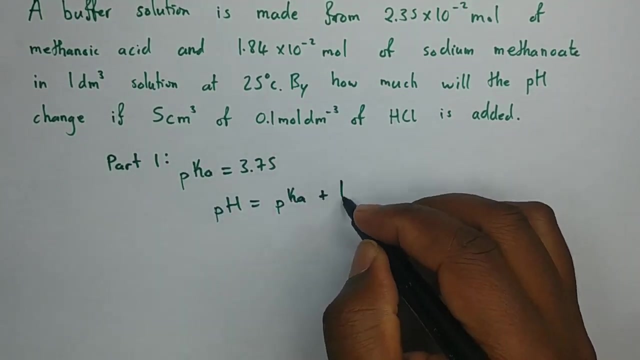 this case is not necessary because we won't be using it. remember, I said we're going to find two separate potential hydrogens, such that when we have the two hydrogens we find the difference. we see if the difference is large or minimal. so let's calculate the pH. we know that the pH is given by the pKa plus the log of A. 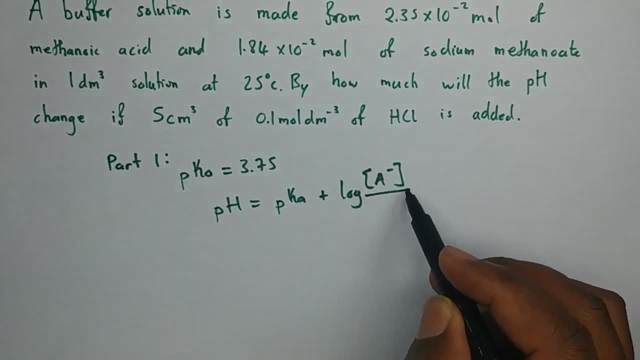 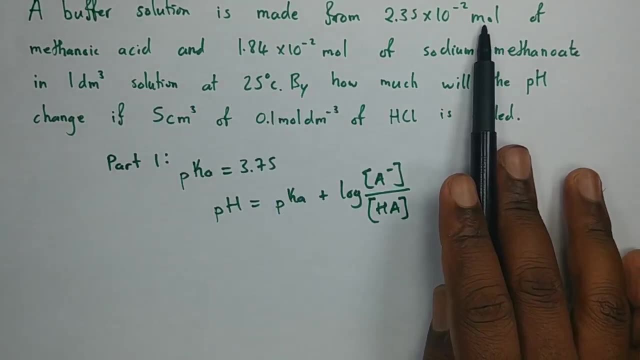 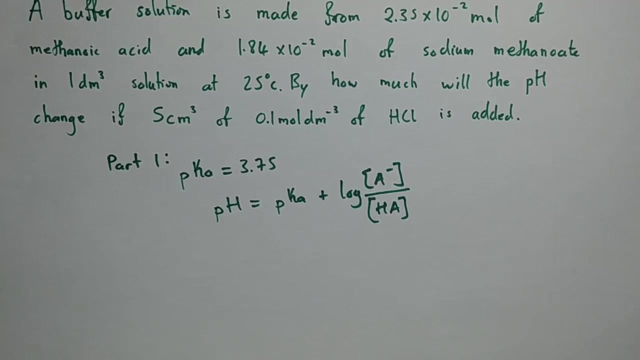 minus, which is a conjugate base divided by a weak acid, which is HA. in the equation we're using moles and not concentration, but one thing we should know is that this can be used as concentrations, simply because these two solutions are in a solution of one cubic decimeter. so 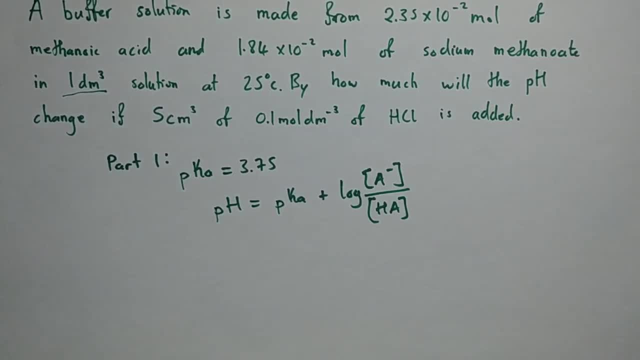 the moles divided by the cubic decimeters will simply give us the concentration. so we ok to assume that is our concentration, meaning that pH will be given us. the pKa in this case is simply 3.75 plus the log of the base. So we need to know which one is our base, which one is our. 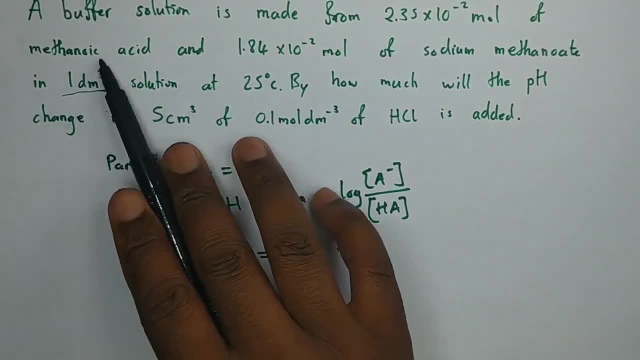 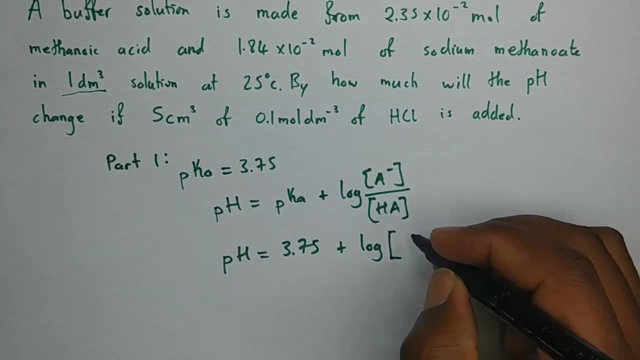 acid. So, according to the equation, the first one here is our acid. so that's the concentration of acid and this is the concentration of the base, meaning that what we're going to have will be 1.84 times 10 to the power negative 2. 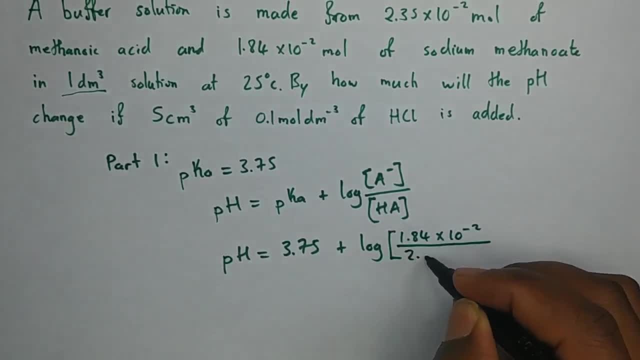 divided by the concentration of the weak acid, which is a 2.35 times 10 to the power negative 2, like that. Okay, so at this stage, if we compute for the pH, we're going to see that our pH, so this plus divide these two and find: 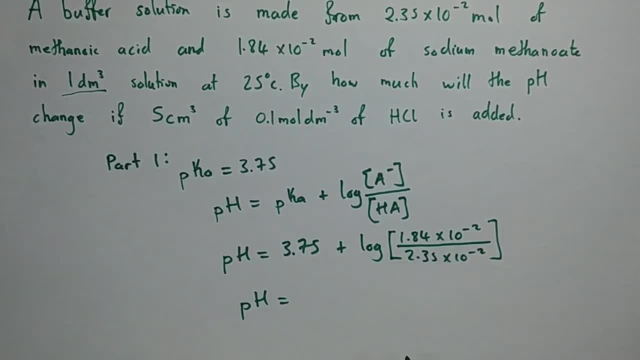 the log of whatever you get, what you're going to have at the end of the day would be 3.64. so that is the first pH of the buffer that we have found. So now, this is the first part. remember we're doing it in parts. 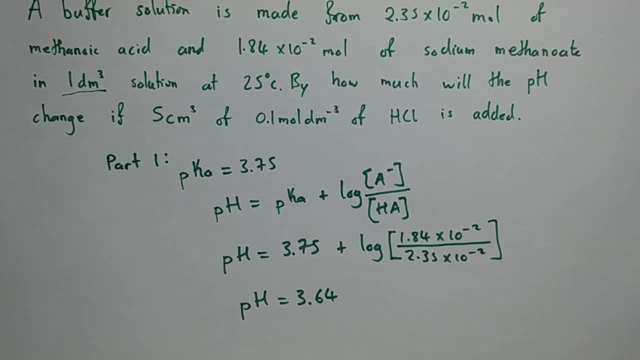 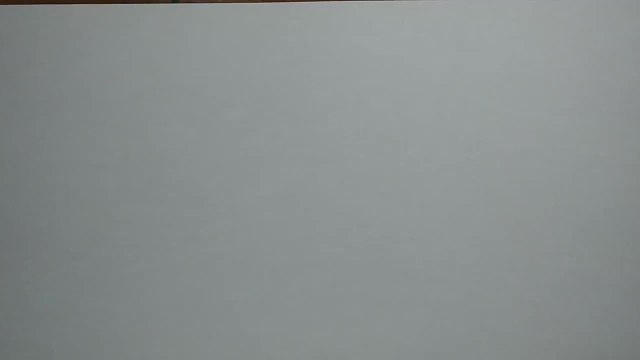 so this is the first part. remember, we're doing it in parts With this pH. I'm going to take it in the other part so that we see how we can find the difference of the two. Okay, so we're going to look at step two now, since we were the previous one. we're looking 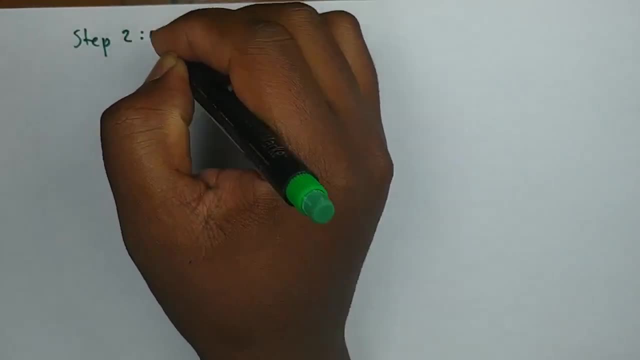 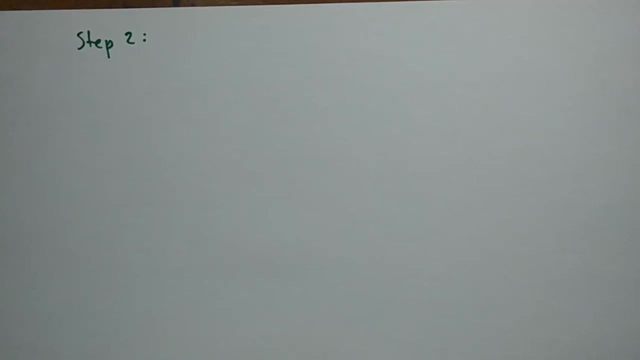 at the step one, So step two. so step two takes place after the strong acid has been added. So we're going to find the moles of the acid. So you can say mole of acid. What we have is 0.1 according to the equation. We have 0.1 and this 0.1 is the concentration. 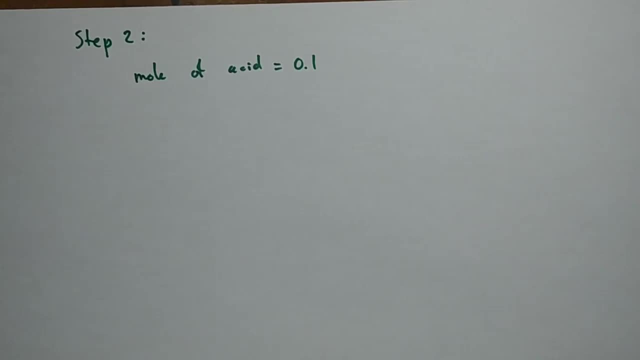 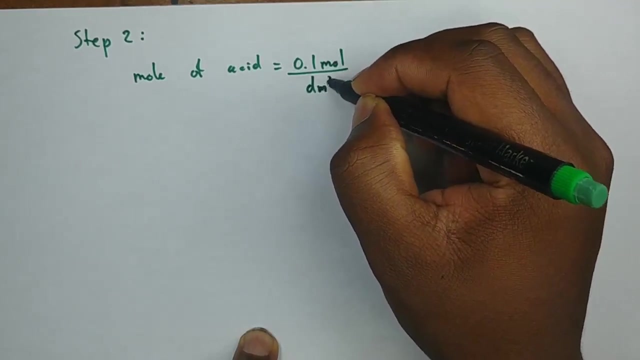 So this 0.1 that we have in the equation can simply be multiplied by the volume. The volume given in the equation, This 0.1 that we have here, is in mole per cubic decimeter. Then the volume that we've been given is five. 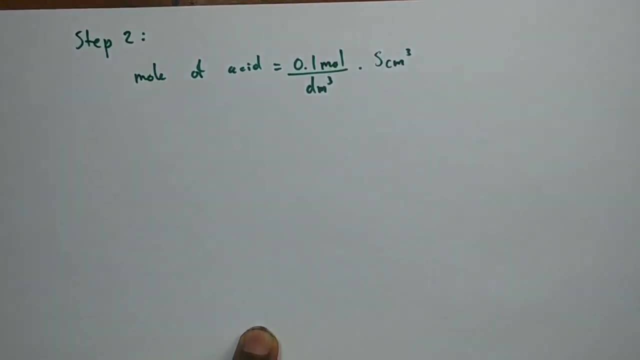 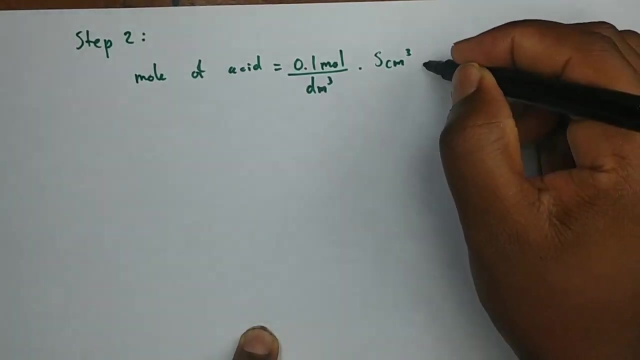 cubic decimeters, like that, But we have to convert this to, sorry, five cubic centimeters, but we have to convert them to cubic decimeters. So this will be given, as one cubic decimeter is equivalent to one thousand cubic centimeters, like that. 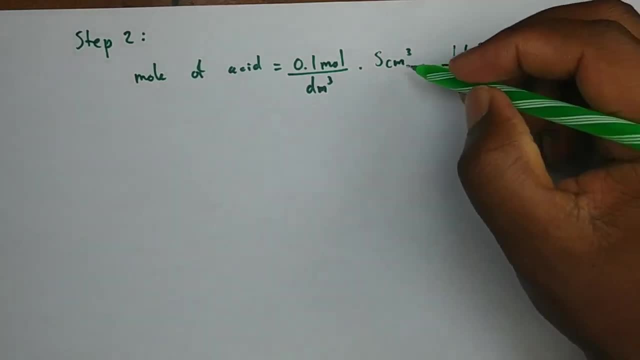 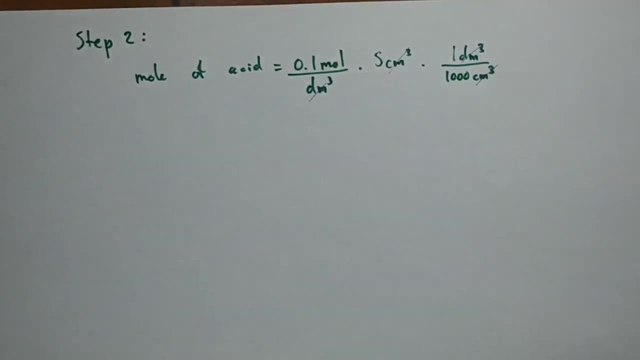 So that at this stage we can see that the centimeter cubic will cancel, the decimeter will cancel. Just remember, it's a number of moles Which, in this case, the number of moles will be equal to five times ten, to the power one. 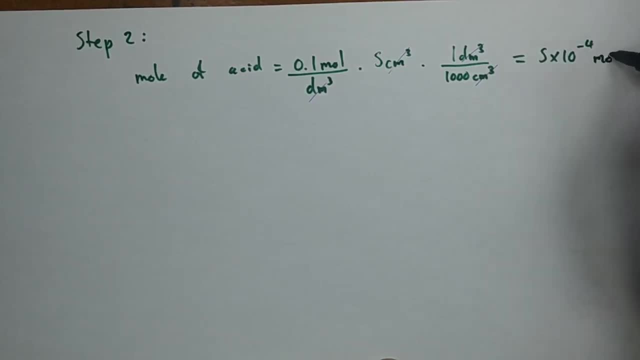 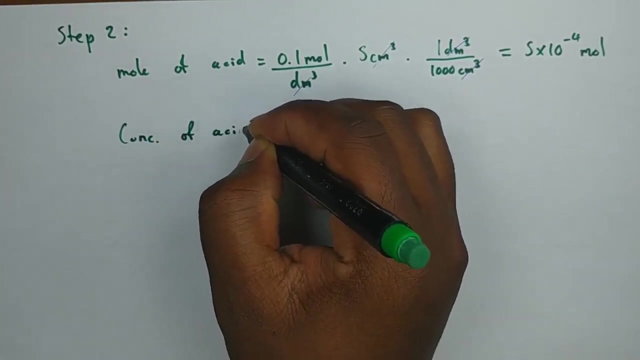 Negative four moles of hydrochloric acid. Okay, So now, with this information, we can transfer it into the process of adding the acid to what we have already. So let's find the concentration, Concentration of acid. So to find the concentration of acid. 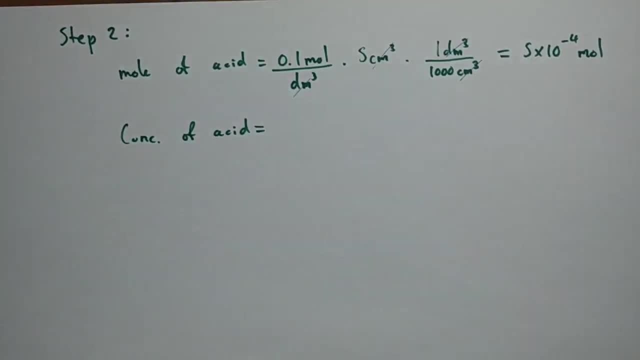 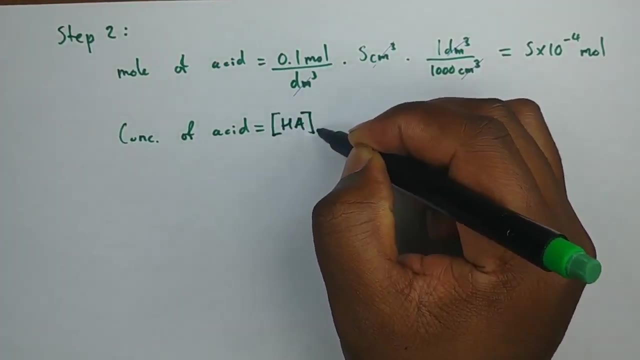 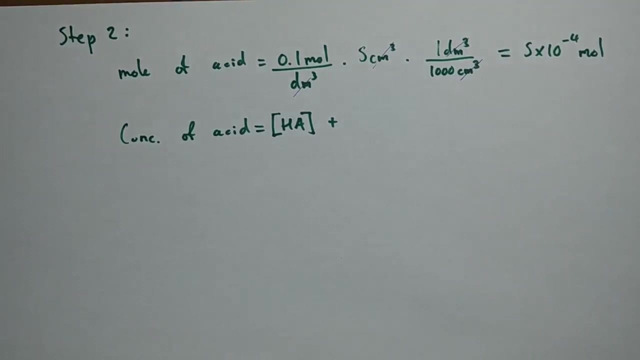 we have to add the concentration of acid that we have already of the weak acid. So we can say the weak acid HA the concentration plus the number of moles of the acid. So why are we adding moles with the concentration? Because the number of moles, like we say the solution, is in one cubic decimeter. 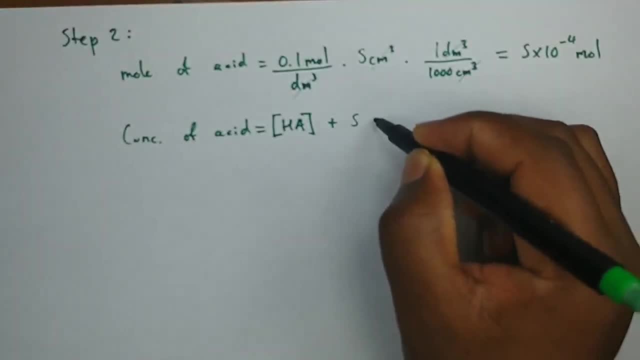 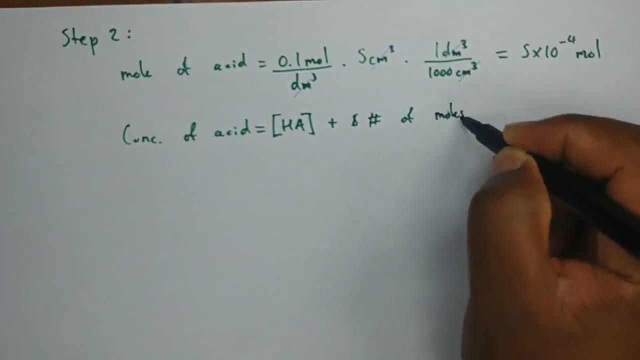 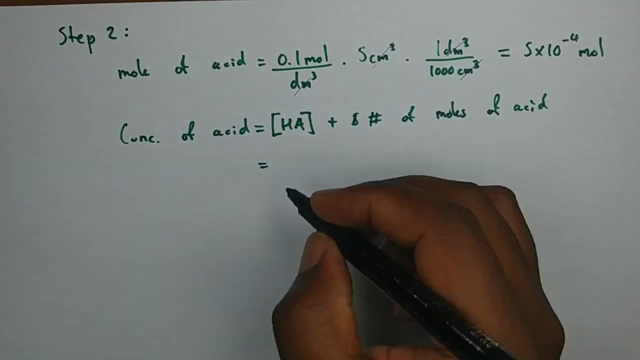 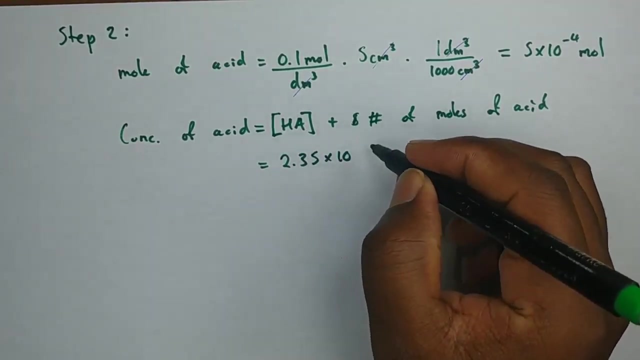 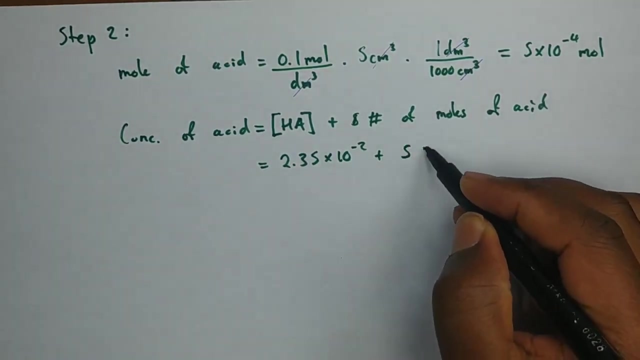 So we can say plus five, or you can just say plus the number of moles of acid. So what is HA? We know that HA is simply 2.35 times ten to the power negative two plus number of moles of the acid that we've just found in this one here, which is five times ten to the power negative four. 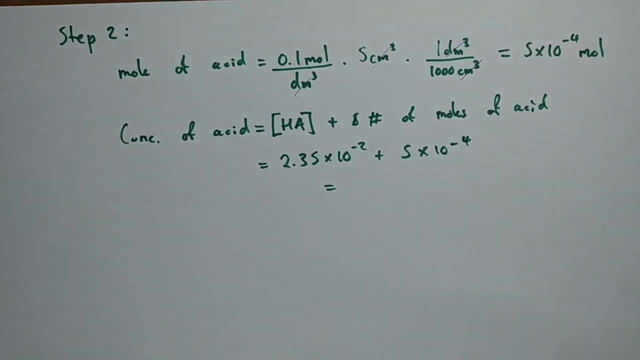 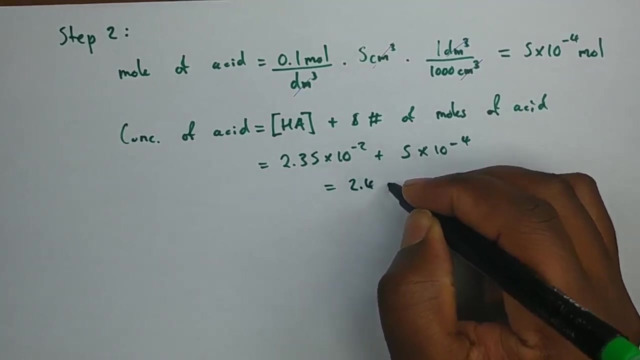 So adding these two values gives us the concentration of acid, gives us the concentration of the acid. So when these two values are added, what we get is simply 2.4 times ten to the power negative two. So 2.4 times ten to the power negative two. Now let's find the concentration of the base. 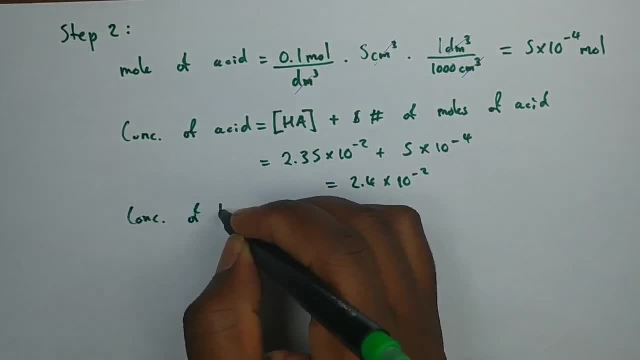 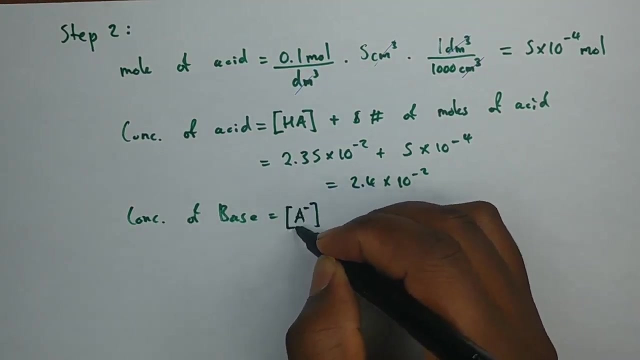 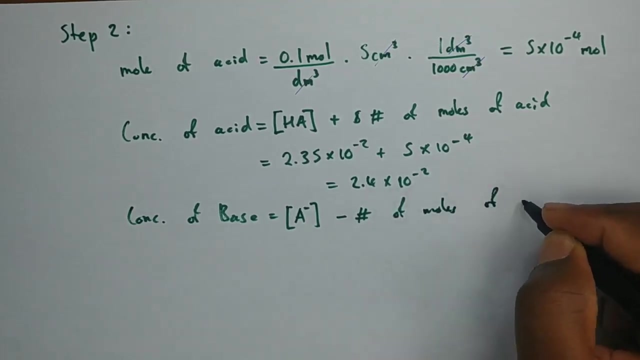 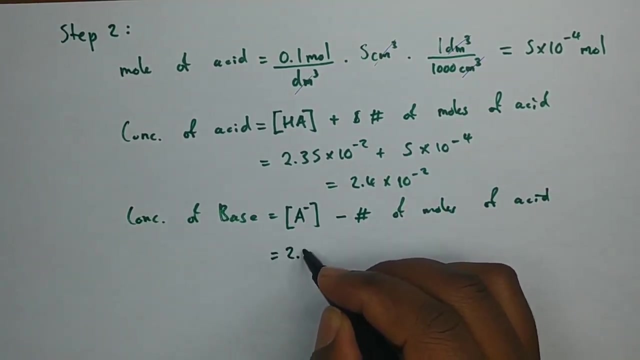 So concentration of base is given by. so, instead of adding the number of moles, we're going to subtract, Because it is a base. So A minus the concentration of the conjugate base, minus the number of moles of the acid, So the concentration of the base we're given 2.3,. 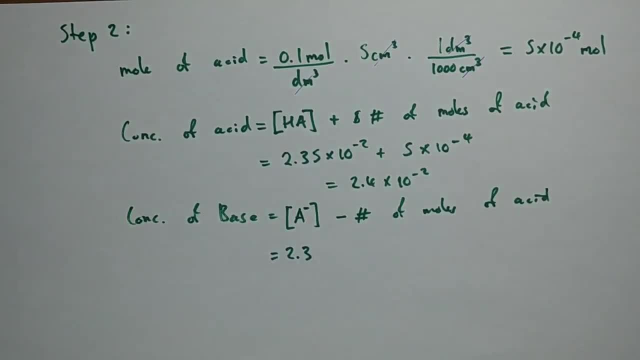 sorry, this is the one for the acid. what we're given for the base was 1.84.. 1.84 times ten to the power negative 2, minus the concentration of the acid, So to the acid we add to the base, we subtract. So this whole thing minus five times ten to the power negative four. 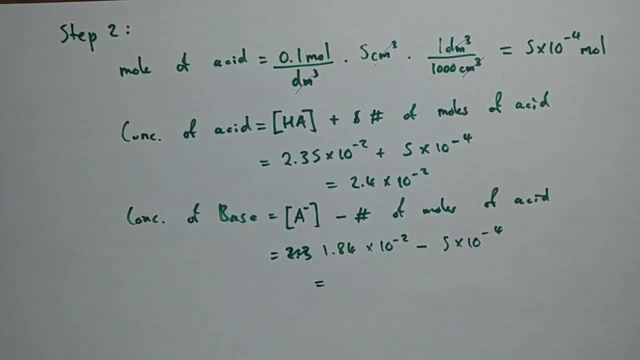 So, subtracting those two, what we're going to get this time around will be 1.79 times ten to the power negative two. So this is what we get. This is the concentration of the acid and this is the concentration of the base. 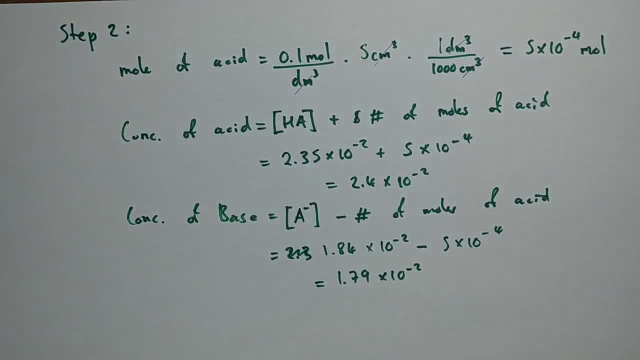 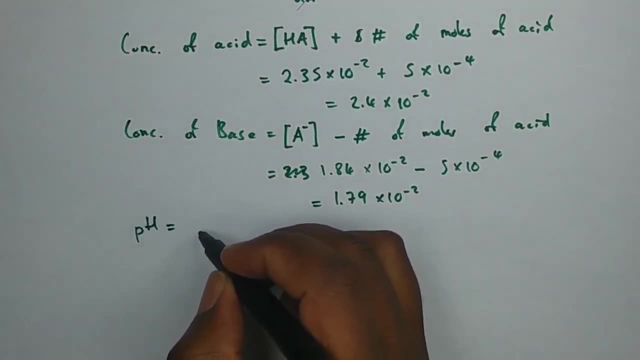 So to find the pH for this part, what I want to do is we're going to say the pH is found by the pKa plus the log of base over acid. So to find the pH, the pKa, we know that the pKa is 3.75.. 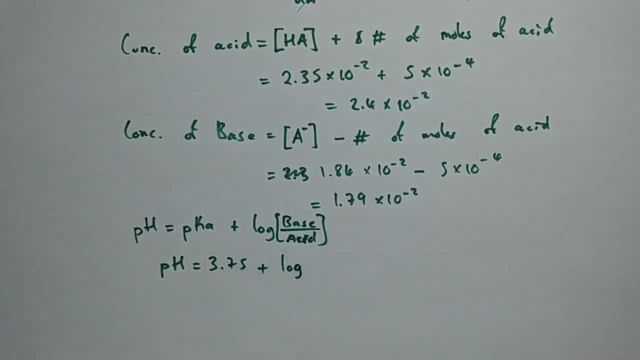 We looked at this in the previous question or in the previous step. Then the log of: for the base, what we have is this one here, because remember, I was saying concentration of the base, which is this one. So for the base we have 1.79 times 10 to the power, negative 2,. 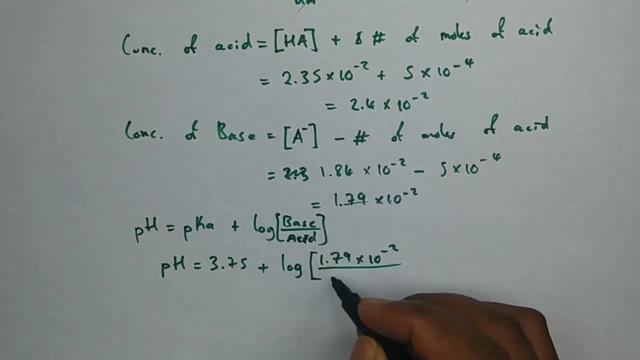 divided by the concentration of the acid, which is this one here, which is 2.4.. 10 to the power negative 2.. So adding these two values, what we're going to get would be 3.64.. So adding these two, what we're getting is 3.62.. 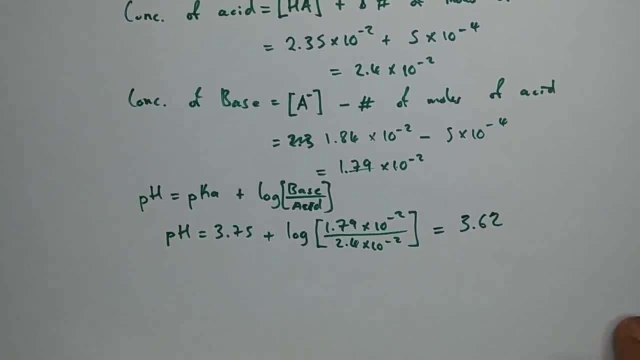 Okay, so now remember. the question requires us to find the change in the pH. So the change in the pH, let's say the change in the pH, is given by the pH final, after adding the acid, minus the pH initial, before adding the acid. 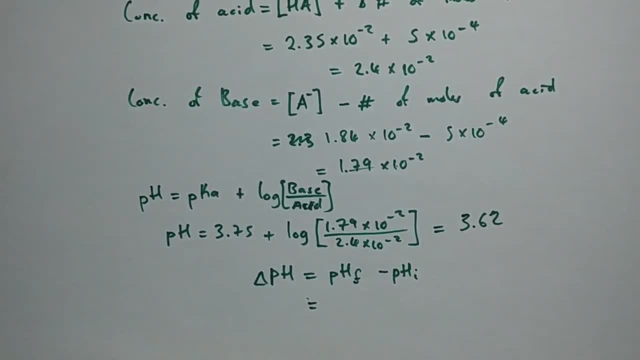 So the final pH that we have, or in this case it's supposed to be initial minus final, that is before adding: yeah, So it's supposed to be initial minus the final. So the initial: we found 3.64 minus the final, which is 3.62.. 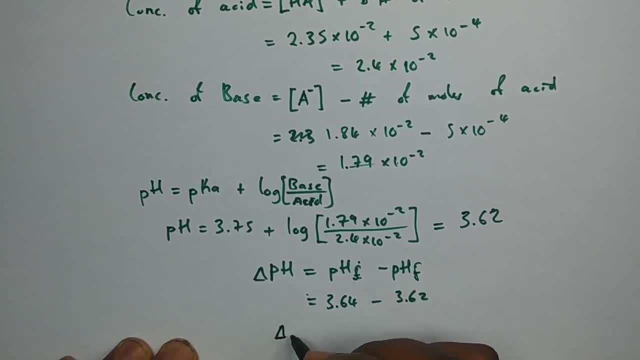 And we see that the difference, or rather the change in pH, is simply equal to 0.02.. Now, this 0.02 is supposed to be a positive value. Why? Because it's supposed to be a positive, small value.